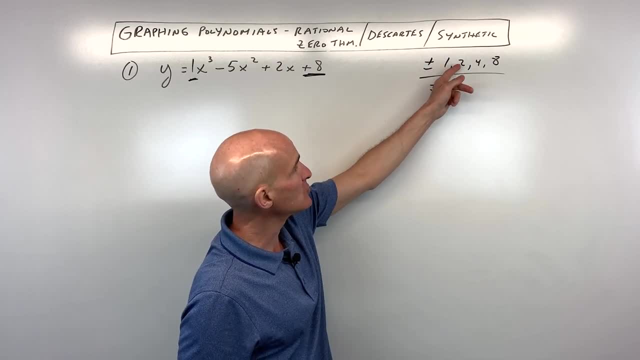 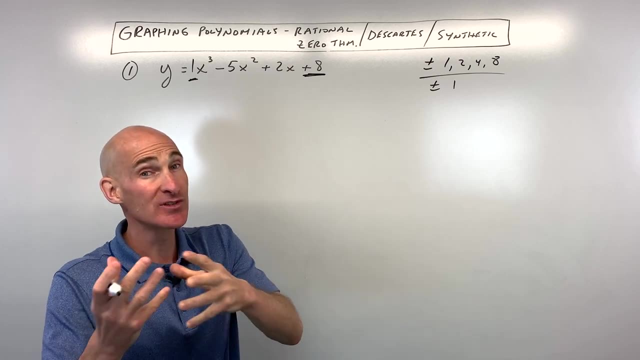 are plus or minus 1.. So it could be 1 over 1,, 2 over 1,, 4 over 1,, 8 over 1, positive or negative. And so what this does is it kind of narrows down the possible zeros, those x-intercepts for us. The next thing we want. 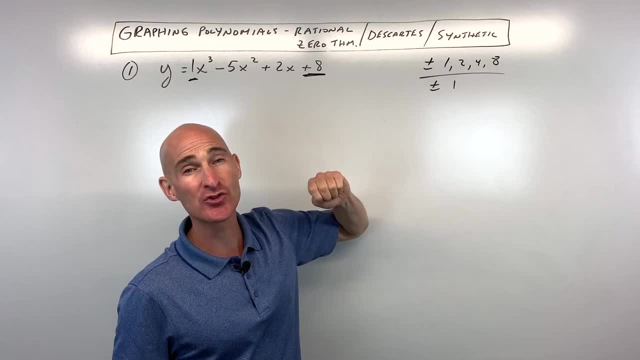 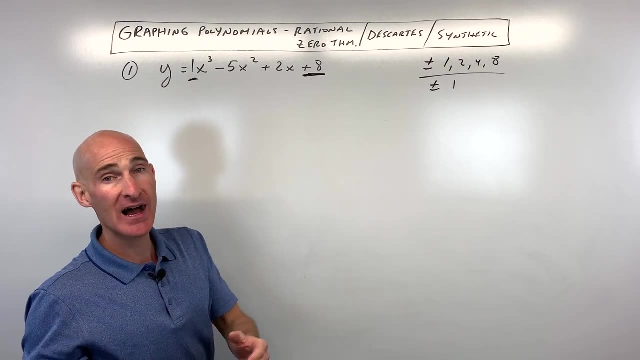 to do is see if we can narrow it down further by using Descartes' rule of sines. So the way Descartes' rule of sines works is we look at the sign changes like positive to negative or negative to positive. that's considered a sign change. So here we have a positive x cubed to negative 5x. 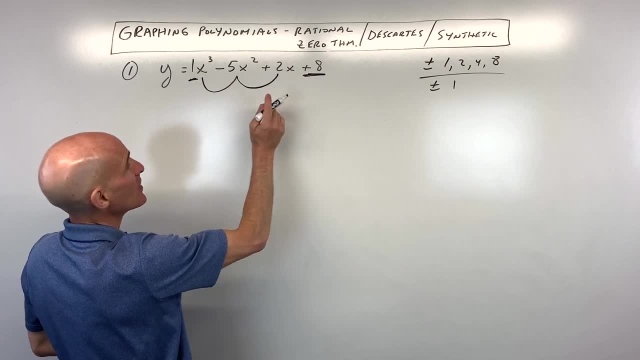 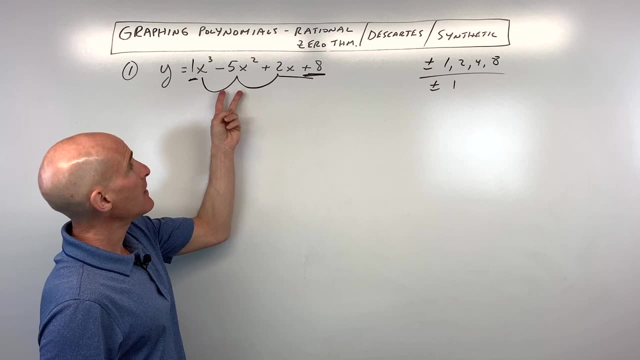 squared, that's 1.. Sign change: Negative: 5x. squared to positive 2x, that's another sign change. Positive 2x to positive 8, that's those are both positive. it didn't change signs, So we have a maximum of 2 positive zeros. 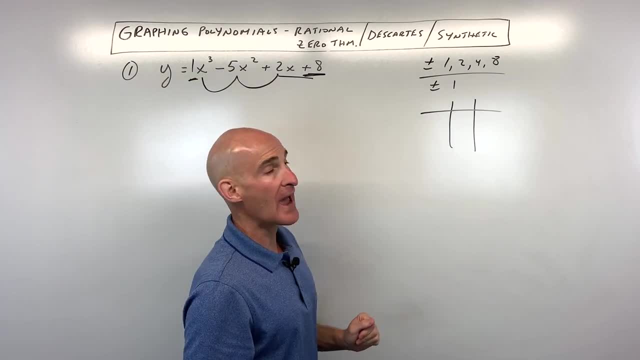 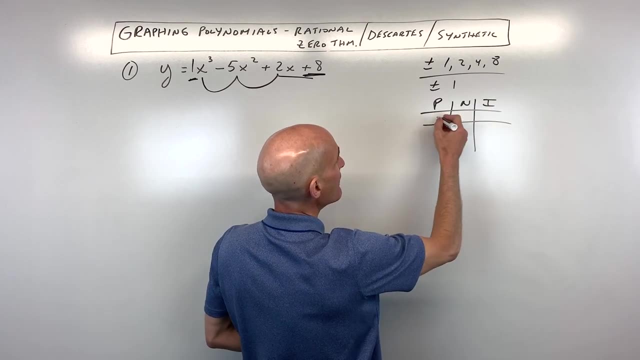 meaning like it's crossing to the right of the y-axis. so positive zeros. So you can make what they call a PNI chart- positive, negative, imaginary- and we're going to have a maximum of 2 positives. Now how about the negative? 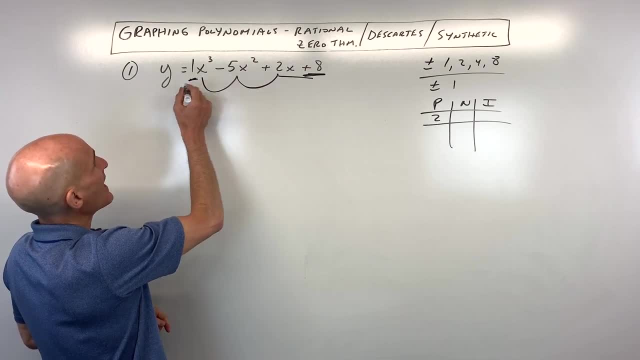 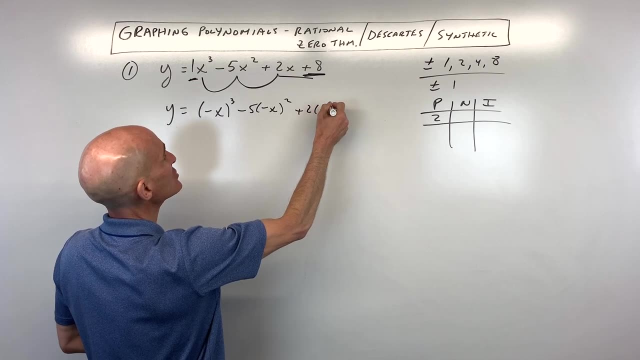 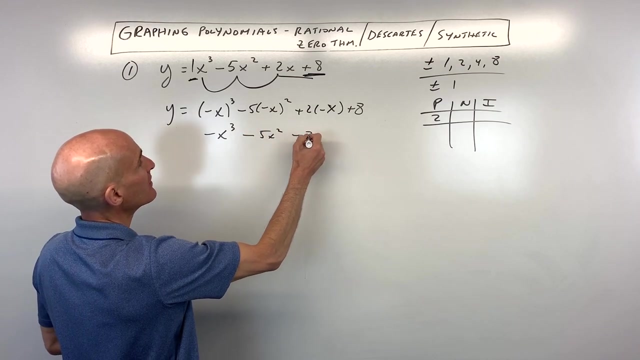 Well, what you can do is you can replace x with negative x, Okay, wherever you see x replaced with negative x. and then what we're going to do is we're going to count the sign changes that occur when we simplify this. So this comes out to negative x cubed, negative 5x squared, negative 2x and positive 8.. 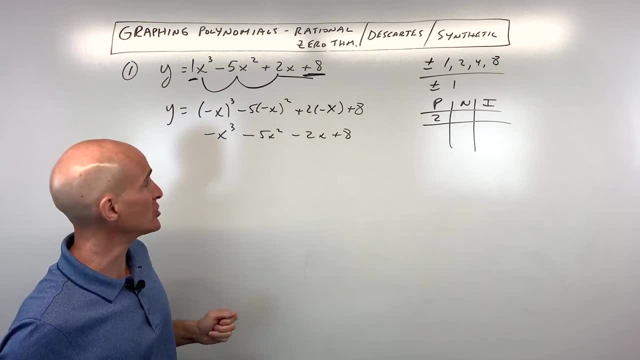 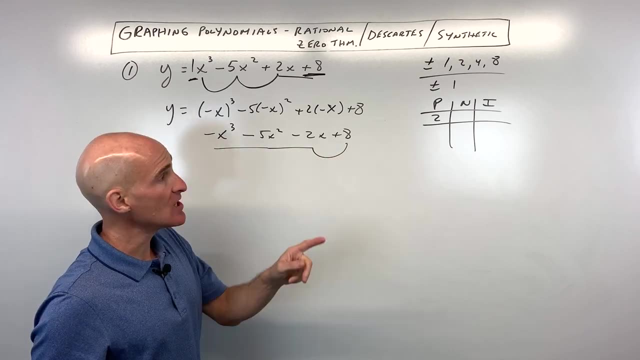 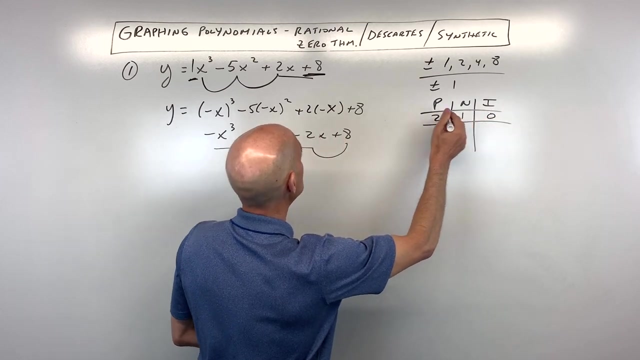 You want to make sure you do your order of operations, the exponents, before you do the multiplication. Now, when we look at the sign changes- negative to negative, negative to negative, negative to positive- that is a sign change. So that means there's a maximum of 1 negative and if you add across here 2 plus 1 plus 0 adds up to 3,. 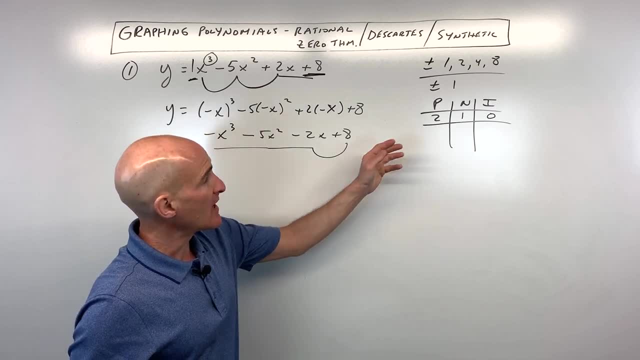 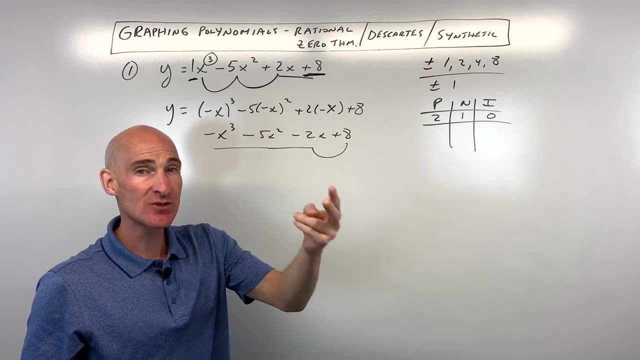 which is our degree of our polynomial. So that's one scenario. Now remember how we said there was a maximum of 2? It could be less than that by an even amount. So you can subtract 2,, 4,, 6,, 8, like that. 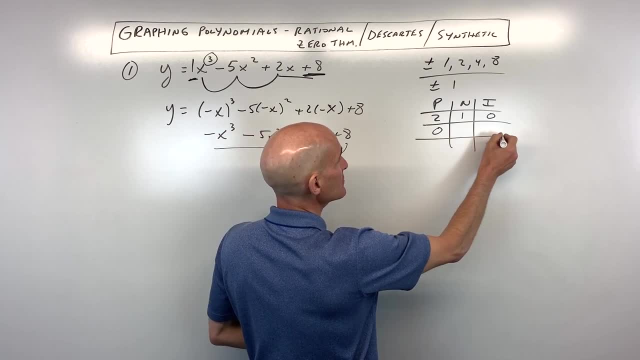 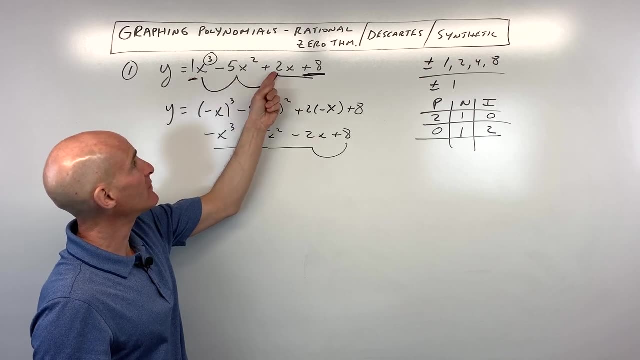 So if I subtract 2 from 2, that could be 0 positives, okay, 1 negative and 2 imaginary. Now when the coefficients are real numbers, see 1, negative 5,, 2, 8, you don't see like 2i or 5i If all the coefficients are real numbers. 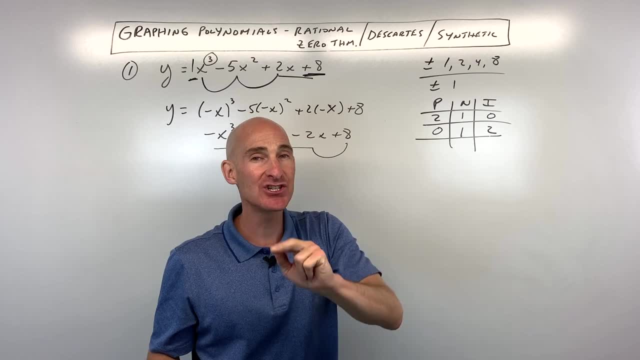 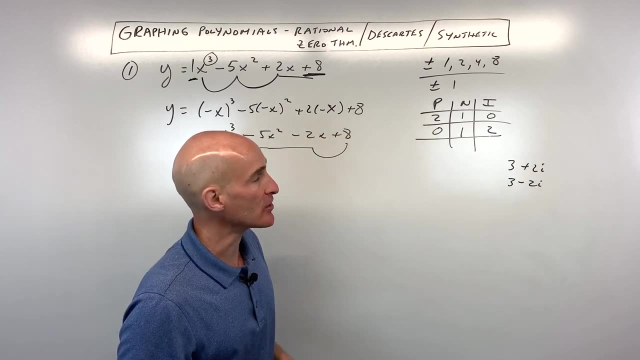 then the imaginary zeros are going to come as conjugate pairs, like a plus bi, like 3 plus 2i, 3 minus 2i. they come together as conjugate pairs. Now what about for the negatives? Could I take 2 away from 1?? 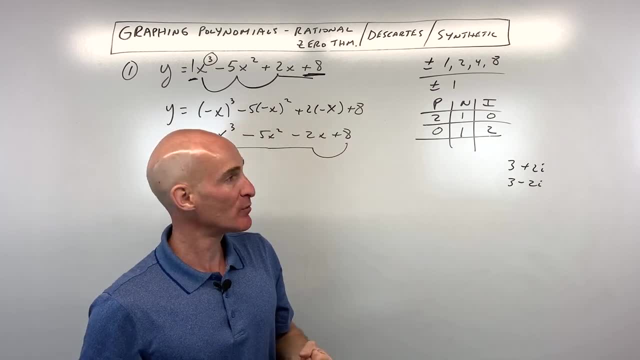 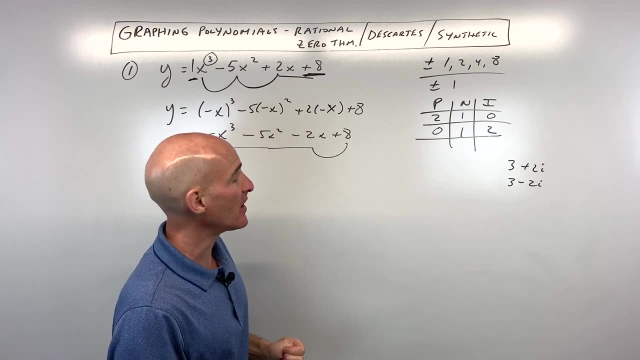 Well, no, because then that would be a negative number of zeros. You can't have a negative number of zeros, So these are the only possibilities for our zeroes. Now you're saying, Mario, how does that help us? Well, when I go to check these, 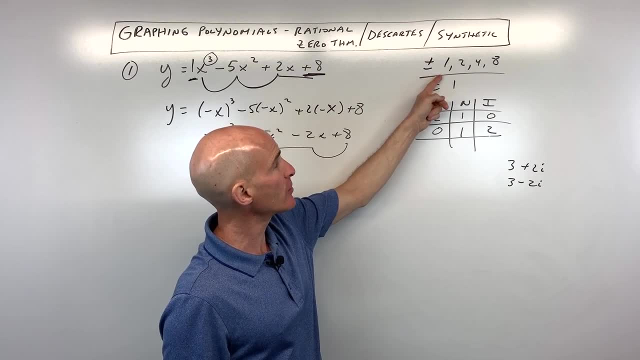 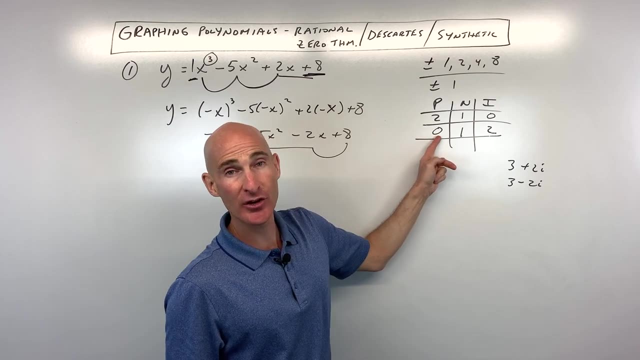 possible zeros here that we found with the rational root theorem or rational zero theorem. I know that there's exactly one negative. If I look for the positives- and it's this scenario here- I might be looking all day and not find them, because there might be none. 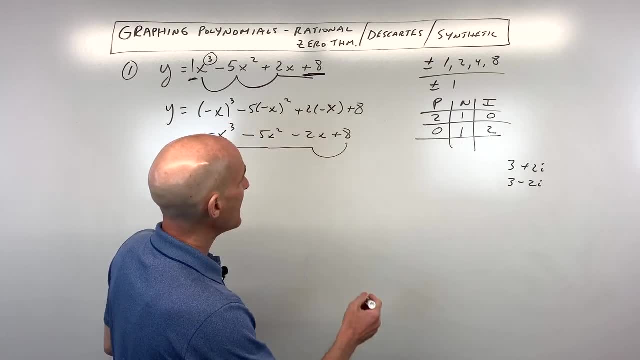 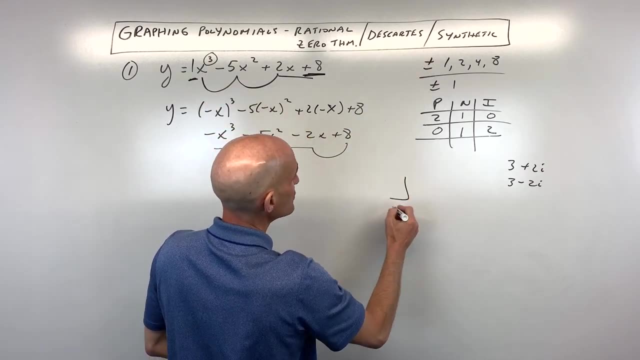 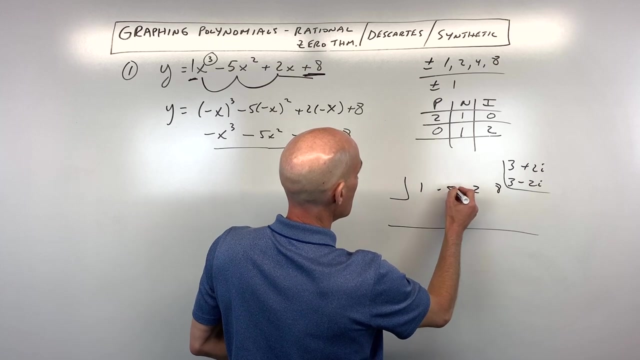 So, to be strategic about this, I might want to go after the negative zero. So, for example, let's go ahead and do our synthetic division. now We want to set it up so that we have 1, negative, 5,, 2, and 8.. 1, negative, 5,, 2, and 8.. Okay, so these are the 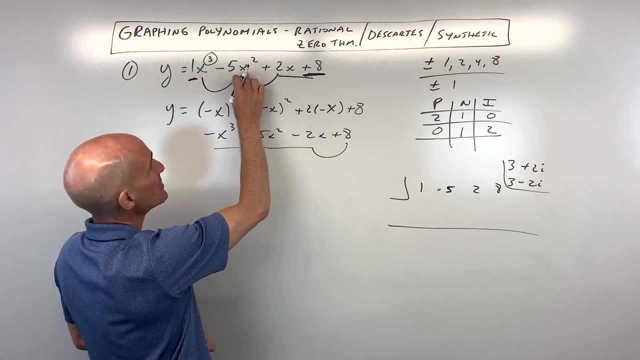 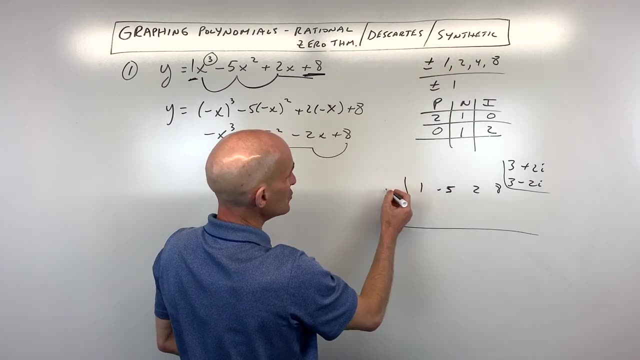 coefficients. Remember, if you skip over any terms, like if it went from x cubed to x, you'd have to put a placeholder of 0 there. but we've got all the terms And then let's test out. say, for example, negative 2.. Okay, so we bring down that first term, we multiply. 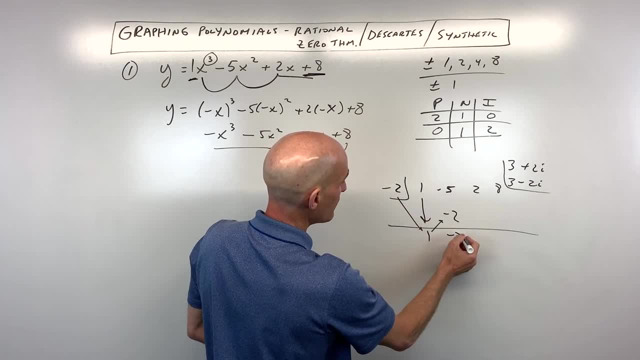 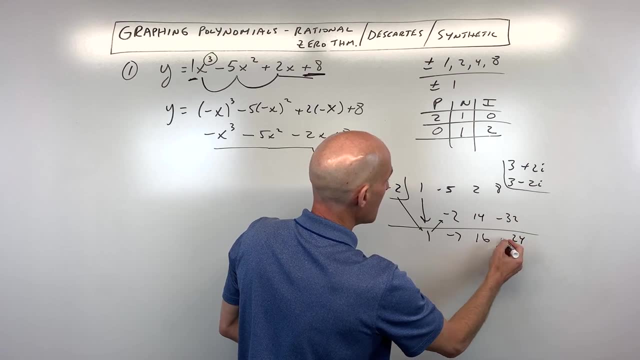 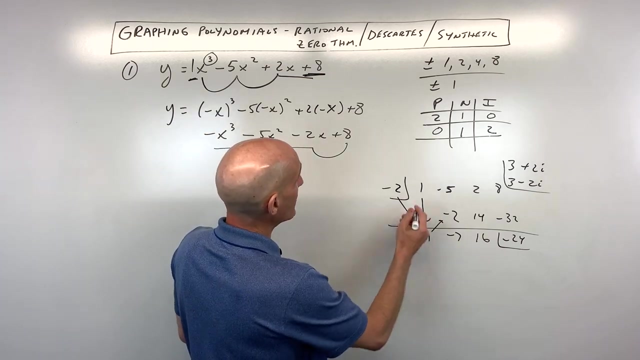 on the diagonal and we add straight down. We multiply on the diagonal, we add straight down, we multiply on the diagonal, we add straight down, and you see how this last number is not 0? That means that negative 2 is not a 0, right, So let's try negative 1.. Okay, 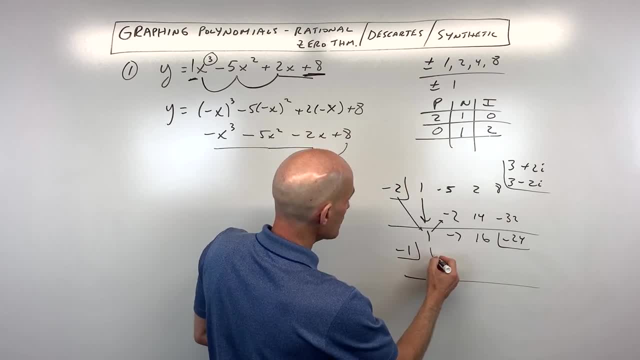 that's one of our possible rational 0s. Start again with our coefficients, which are coming right here: 1, negative 5, 2, and 8.. Let's drop down that first number. multiply on the diagonal. add straight down. multiply on the diagonal. add straight down. multiply on the. 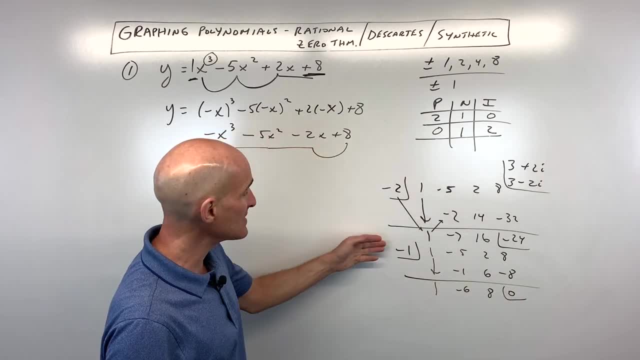 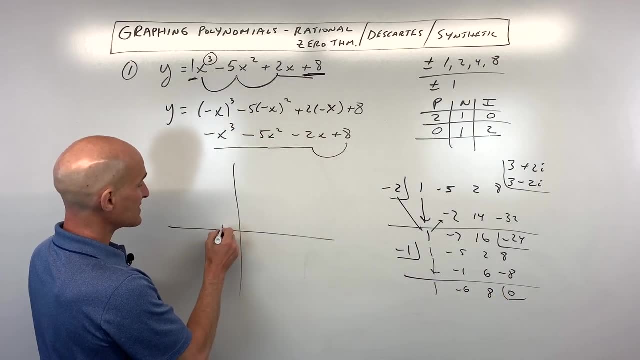 diagonal. add straight down Here we are getting 0 remainder, which means that negative 1 is a 0. So what that means graphically here is it's going to cross the x-axis right here at negative 1.. That's our. 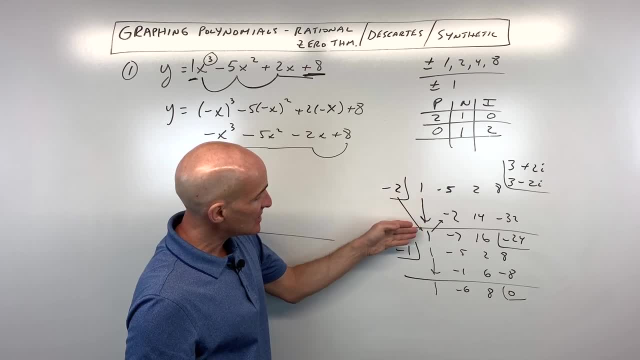 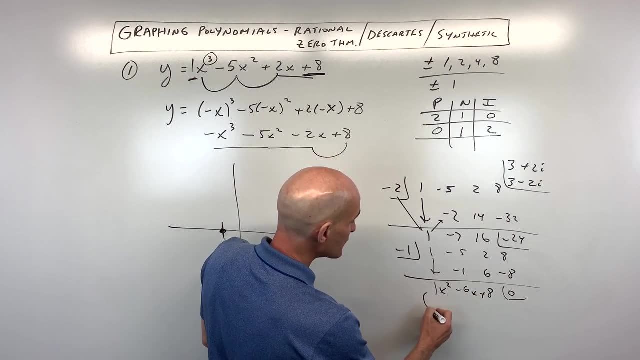 0.. But now when you do the synthetic division, it takes you down 1 degree, So it takes you from x cubed down to x squared, and we can factor this further. now This is going to be x minus 4,, x minus 2, and then this was like x plus 1.. So when you set this to 0,, 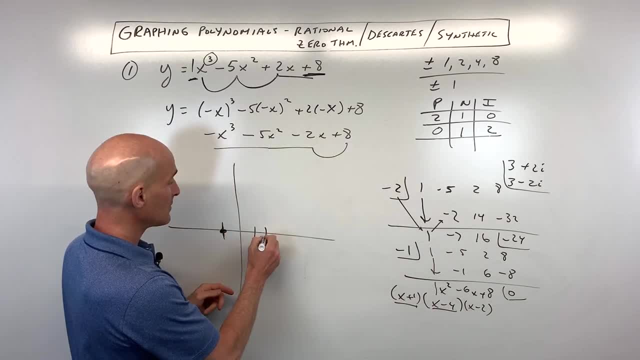 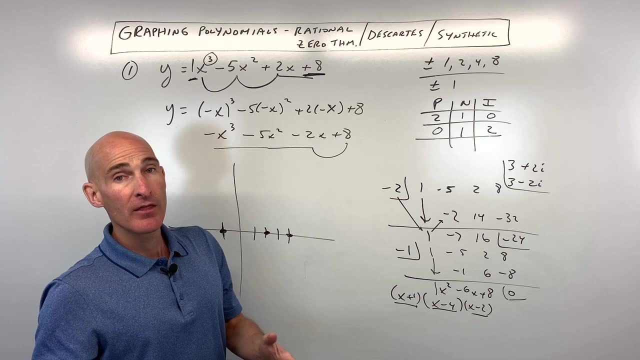 you get negative 1.. When you set this to 0, you get 4.. So it's crossing here at 4.. And when you set this factor to 0, you get 2.. So now we found our 0s. The only thing we need to do now is analyze. is the graph going? 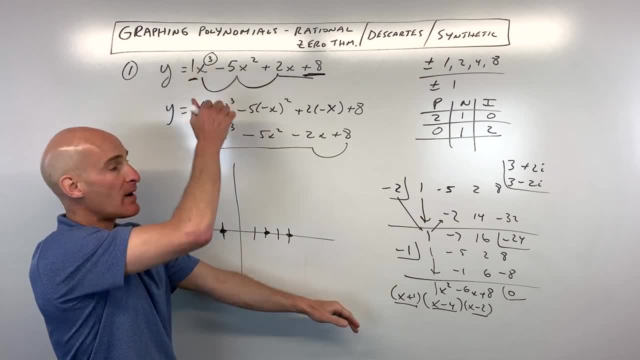 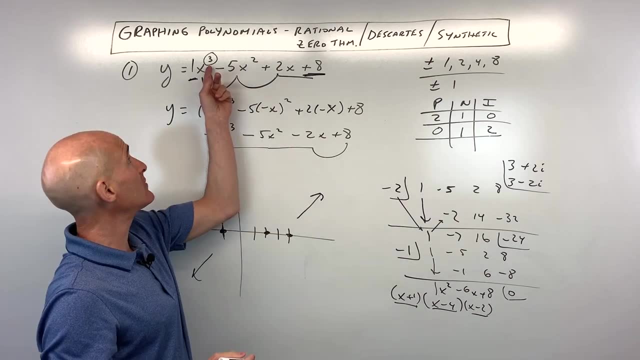 up to the right or down to the right. Well, the leading coefficient is positive, so we know it's going up to the right. The degree is odd, so it's going the opposite way to the left. If it was an even degree, they're either going to both be going up or both going. 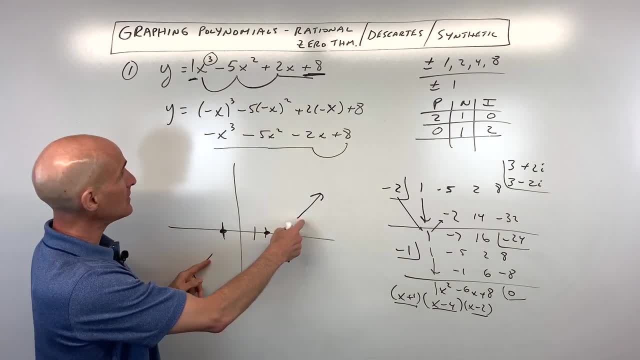 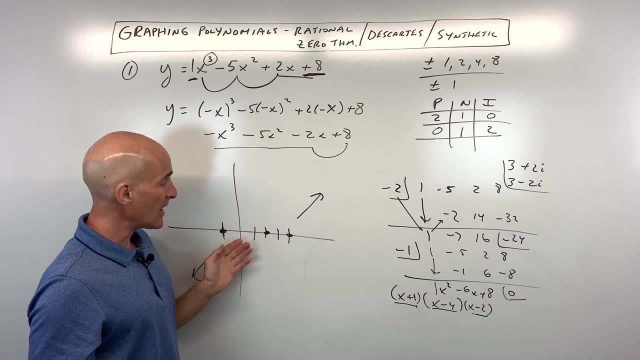 down. They're going the same direction But, odd, we go opposite And it looks like that the 0s all occurred once. We didn't have any multiplicities. It's not like a negative 1 occurred twice or three times, They all just occurred once, So that 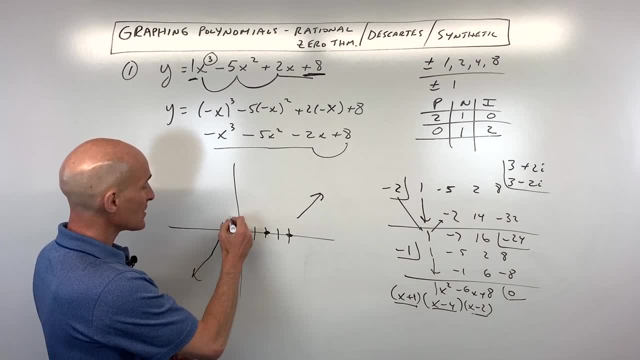 means that when it crosses at these points, it's going to cross just like a line. If it was a multiplicity of 2, it would bounce. If it was a multiplicity of 3, it would have that x cubed shape. But these are all occurring once, so it's going to have this where it. 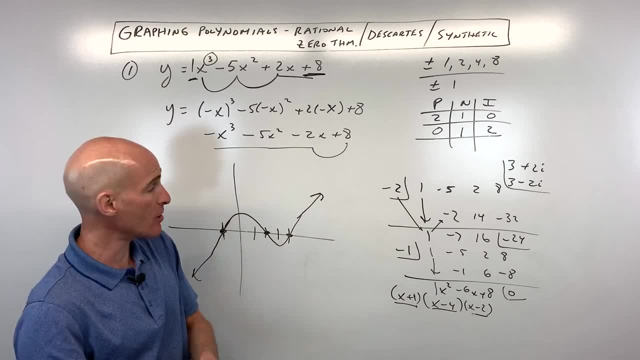 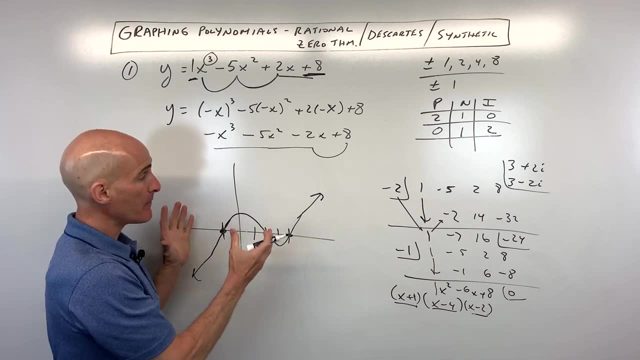 goes straight through at each of those x intercepts. Now, the only thing that's missing here. we could plot some points in between these 0s to get an idea about how high it goes or how low it goes, to get a better sketch. But 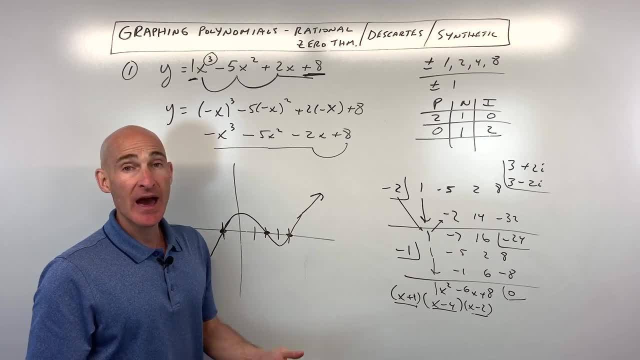 overall, this is a pretty good sketch of our graph and you got it. Let's look at number 2, where we get into another example. Before we jump into example number 2,, if you're new to the channel and we're meeting for the 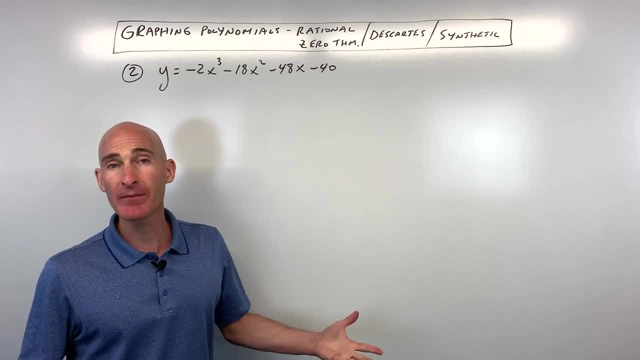 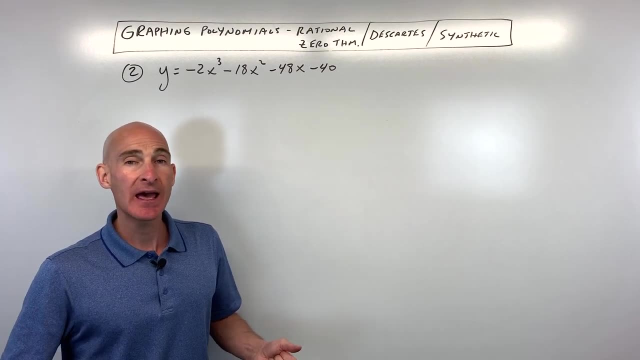 first time. my name is Mario of Mario's Math Tutoring. I'm a full-time math tutor. I work with students every day And what I do is I take what works the best and the quickest and the easiest for students and I take them and I try to condense it down and put it into. 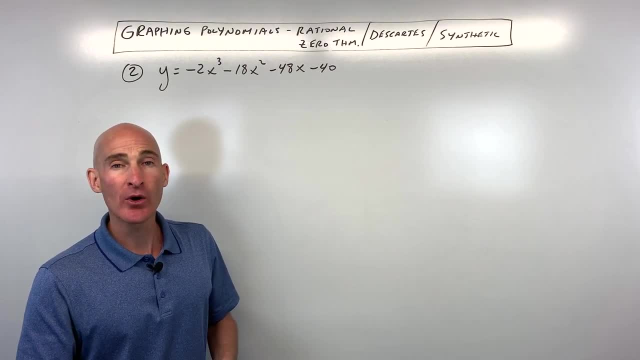 these lessons So you can benefit from my techniques. You can benefit from my tutoring as well. So my goal for the channel is to make learning math less stressful, so you can raise your grade, pass your class and go on to pursue your dreams. 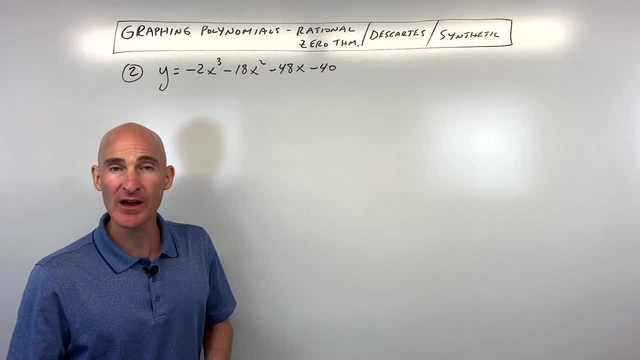 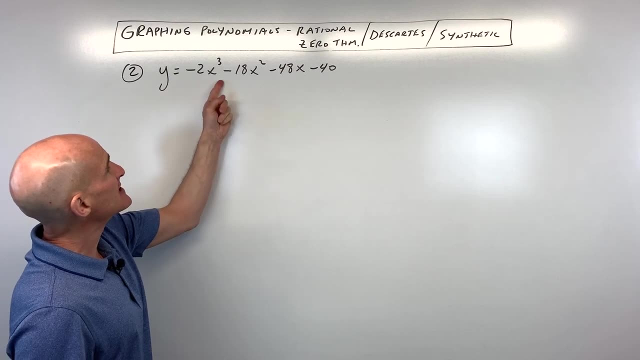 If that's something you're interested in, check out more math videos on my Mario's Math Tutoring YouTube channel. But let's jump into number 2 and get some more practice with these problems. The first thing I would do is I'd see if I can factor this: 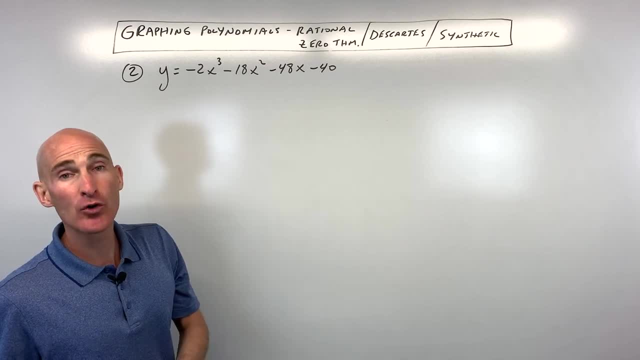 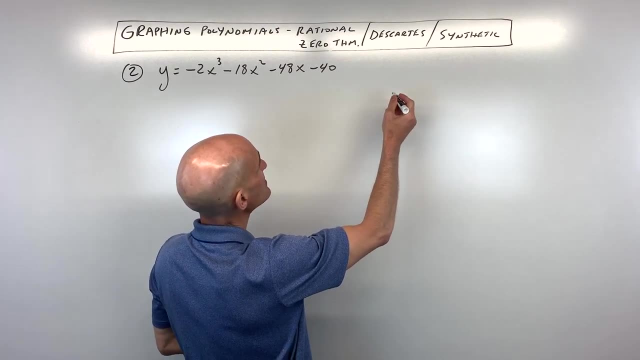 You know, I would try to factor it. If it can't factor it, then I would go to the Rational Zero Theorem. And so, in this case, let's just go ahead and do the Rational Zero Theorem, since that's what we're practicing. 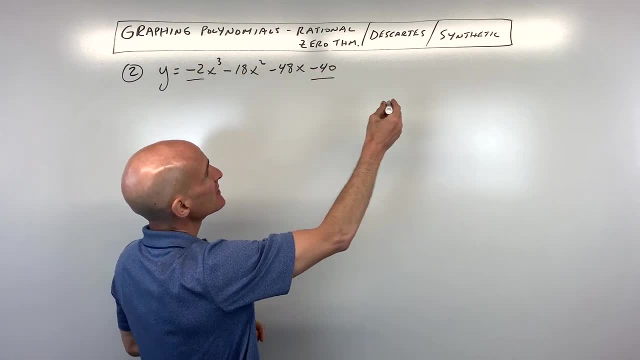 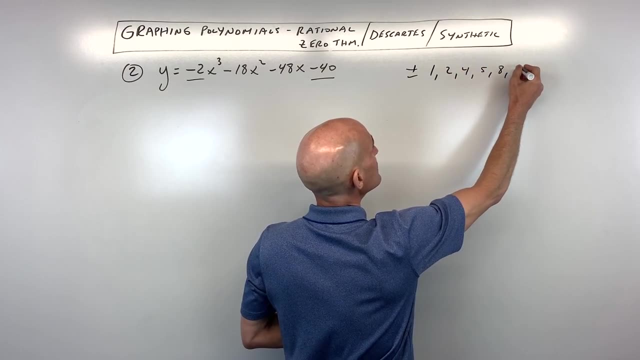 We take all the factors of the constant divided by all the factors of the leading coefficient, So that would be plus or minus 1,, 2,, 4,, 5,, 8, what is that? 10,, 20, and 40, all divided. 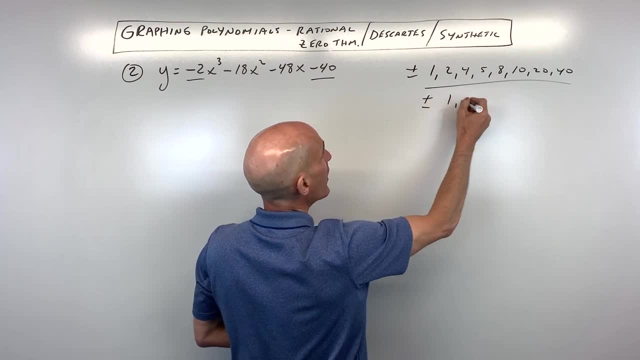 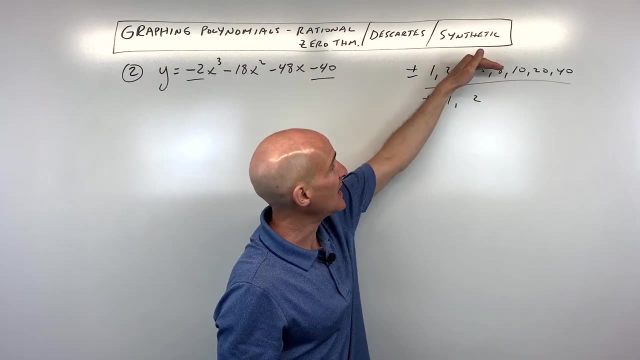 by plus or minus the factors of the leading coefficient, which would be 1 or 2.. So, for example, it could be like 1 half or 5 halves. you know positive or negative any of those combinations, any numerator divided by any of these denominators. here. 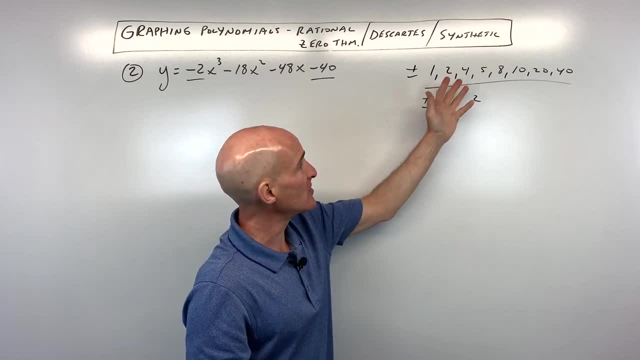 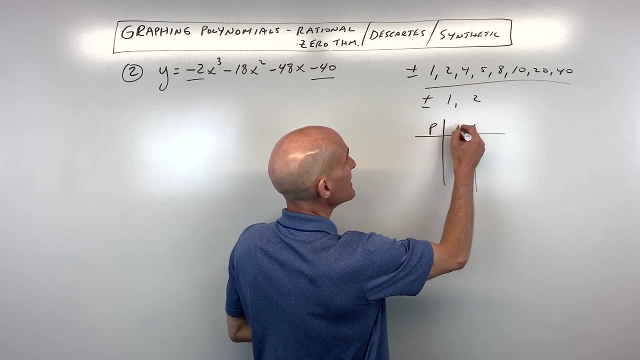 So then let's go to D. We're going to use Descartes' Rule of Science to see if we can narrow down, because there's a lot of zeros here, right? So what I would do is I would make a P&I chart- positive, negative, imaginary- to get an idea. 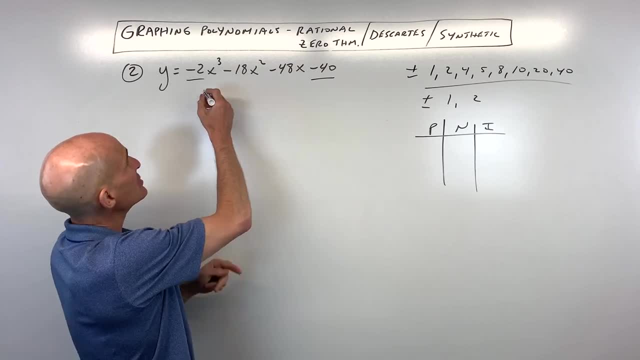 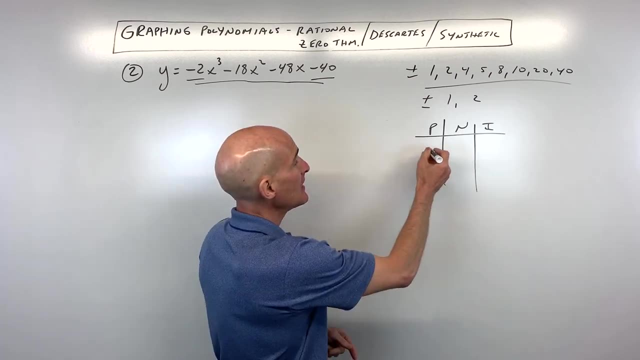 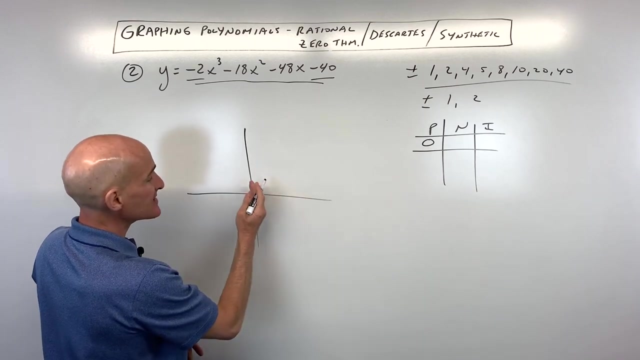 what the possibilities are. So we want to check the sign changes. We've got negative to negative, negative to negative, negative to negative, So it doesn't change signs at all. So there's going to be a maximum of zero positive zeros. meaning when we go to graph this, it's: 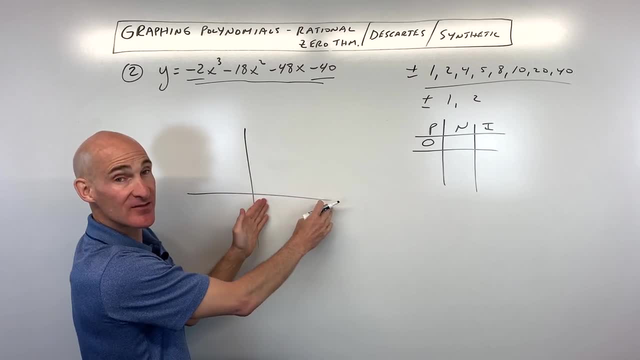 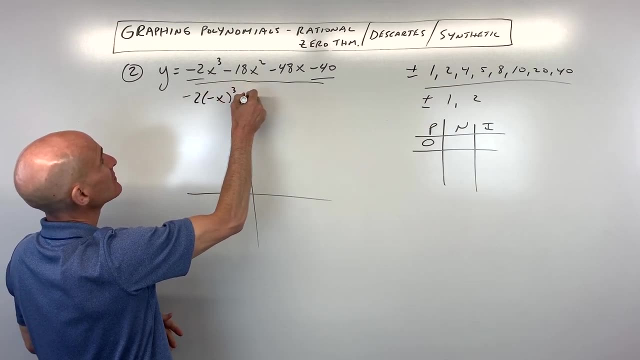 not going to cross over here. to the right of the y-axis, There's no positive zeros. If you want to find the negative ones, what you do is replace x with negative x. Okay, so wherever you see x, you're replacing that with negative x. 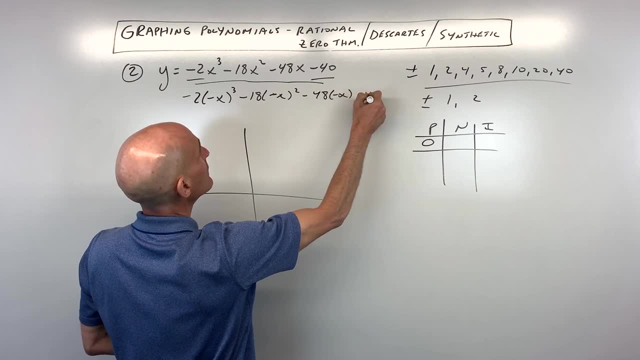 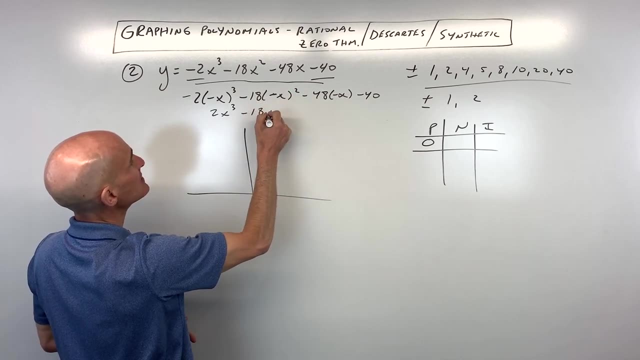 And then what you want to do is you want to simplify that down, And so this gives you negative x cubed times. negative 2 is positive 2x cubed. This gives you x squared. That's negative. 18x squared, This is positive 48x. 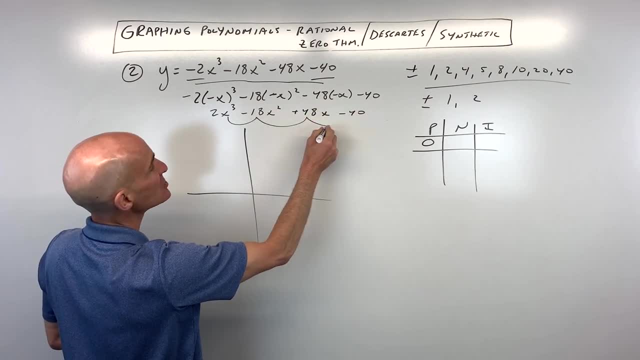 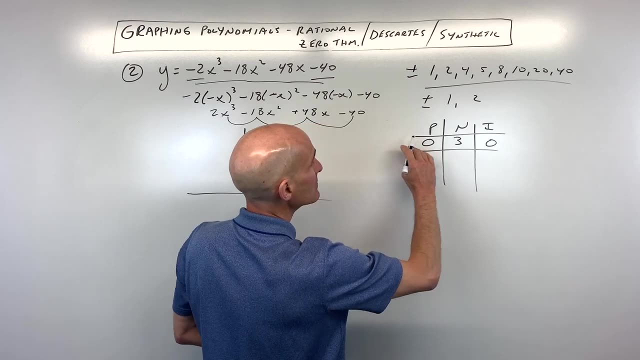 This is negative 40. So now we have one sign change, two sign changes, three sign changes. So that means there's a maximum of three negatives and you can see the zero plus three plus zero is three, It's a third degree. 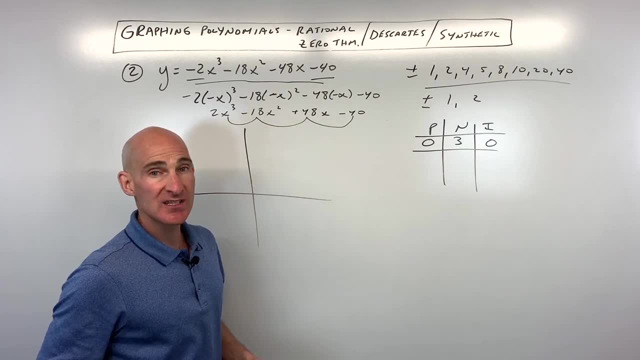 Or remember. these can always go down by an even amount like 2, 4,, 6, 8.. You can subtract 2, 4,, 6, 8, an even number, So it could be zero, one and two imaginary. 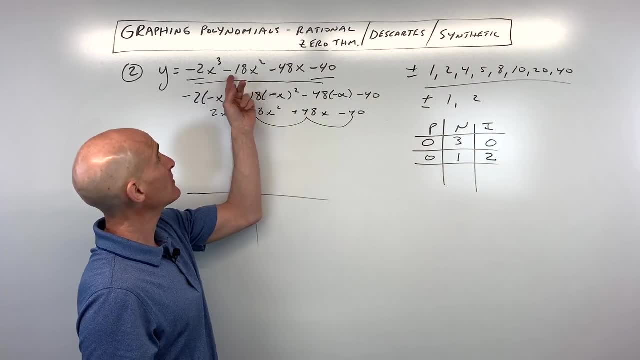 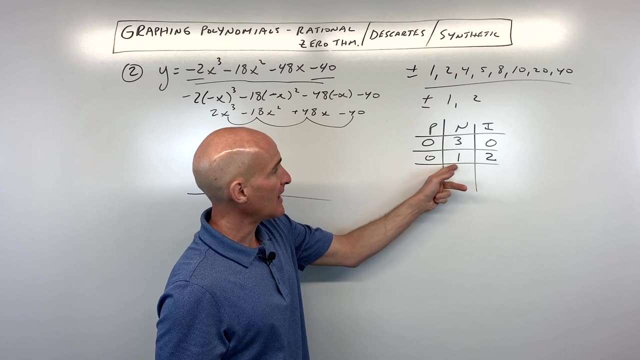 Again, remember the imaginary. come as conjugate pairs if the coefficients are real. You don't see any. i's up there. We can't subtract two Again. that would put us into the negative territory. You can't have a negative number. 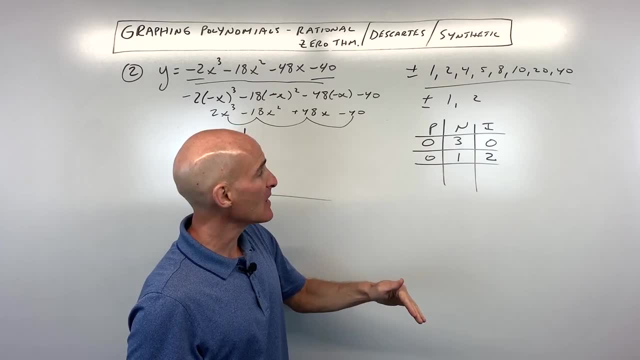 We can't have a negative number of zeros. This one's already at zero. We can't go lower than that. So these are our only possibilities. So you say: well, how does that help us, Mario? Well, we know there's no positives. 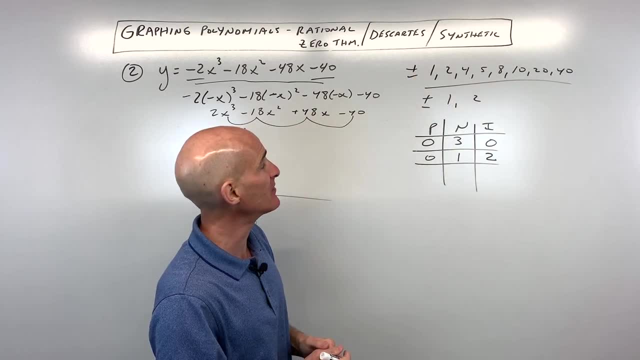 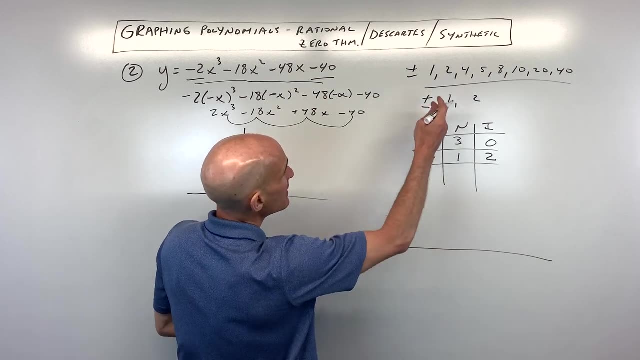 So that already cuts our work down by half. right, We don't have to check any of the positive ones, just the negative ones. OK, so great. So let's go ahead and do our synthetic division. Let's pick a combination of a numerator and denominator. 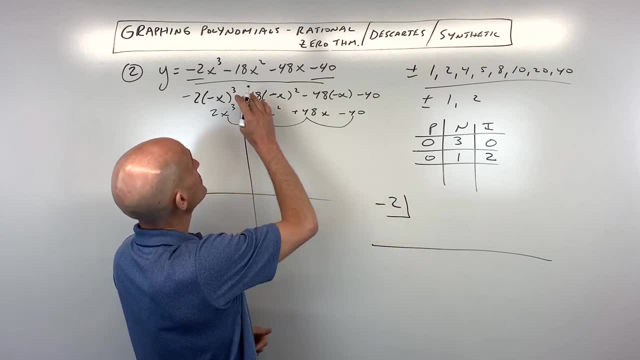 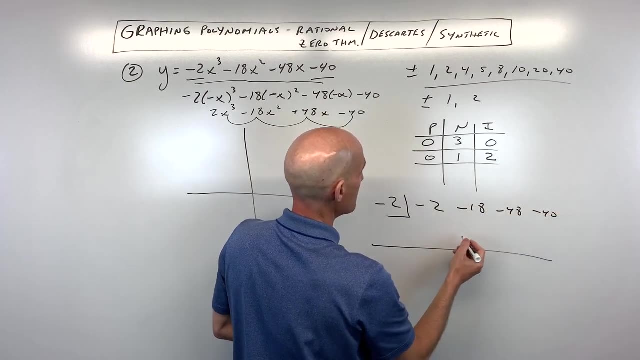 We're going to make it negative, Let's go for negative 2.. OK, so we're going to take our coefficients. We have negative 2, negative 18.. Negative 48 and negative 40. We're not missing any terms, so we don't have to put any zeros for placeholders. 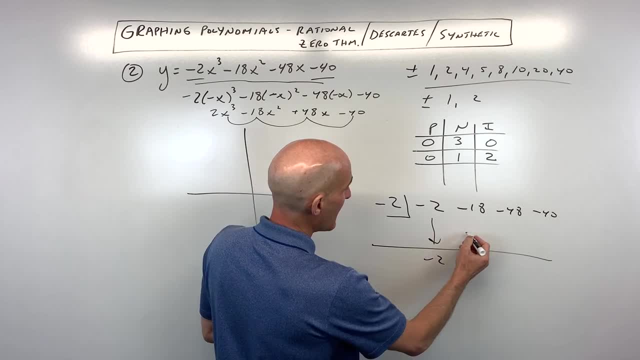 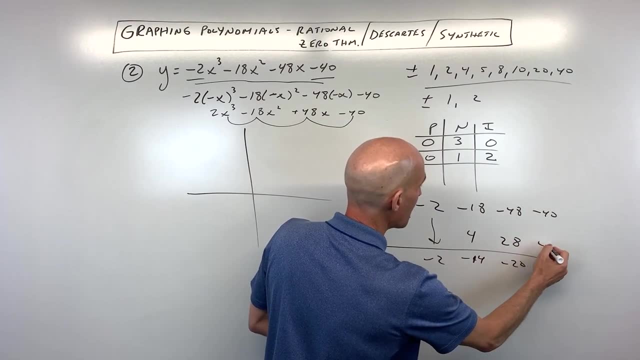 We just have to drop down that first term. multiply on the diagonal- add straight down. multiply on the diagonal- add straight down. multiply on the diagonal- add straight down. Now it came out to zero. so that tells us that negative 2 is a zero. 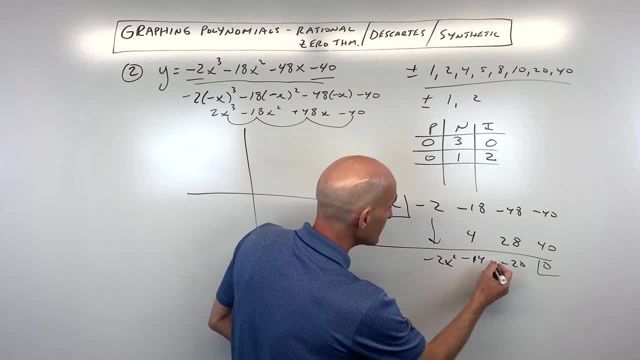 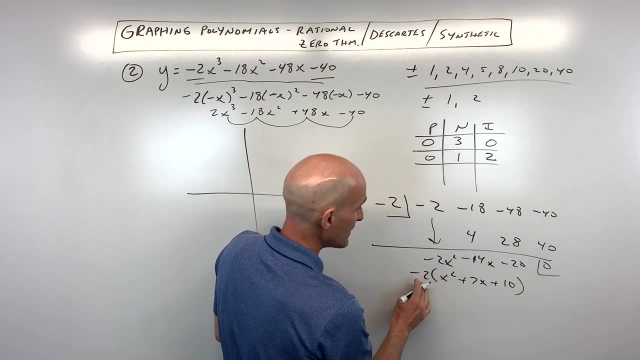 It also brings us down from x cubed to x squared, And so now we can see if we can factor this A little bit further here. So I factored out a negative 2, that was our greatest common factor, and we can factor. 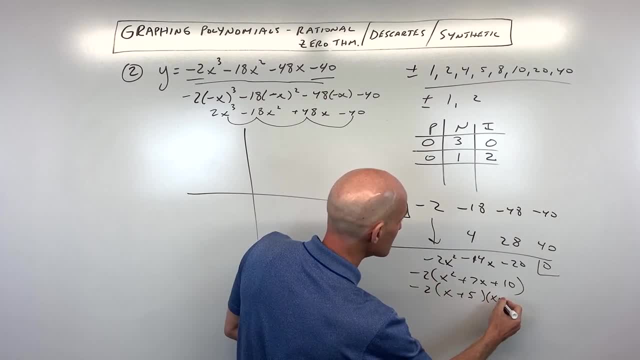 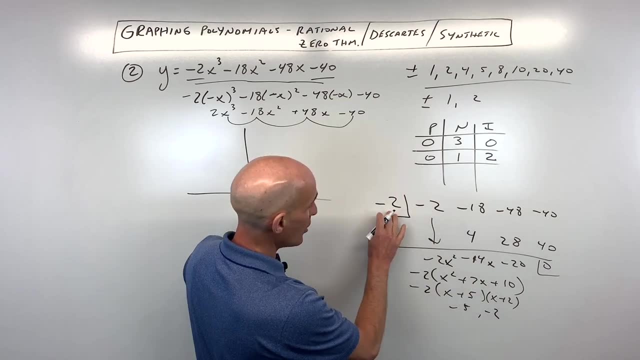 this a little bit further: X plus 5 times x plus 2 gives us back this: and if we set these factors to zero, we get negative 5,, negative 2, and we also had negative 2.. Now this is interesting. 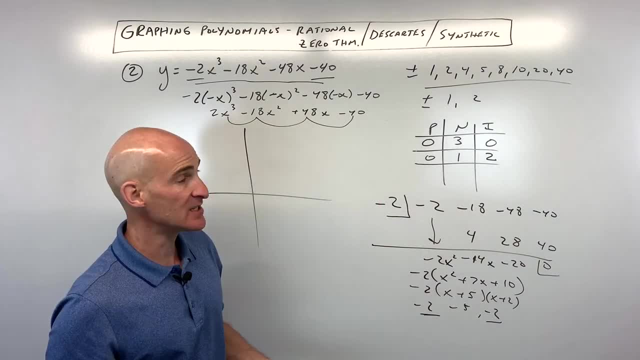 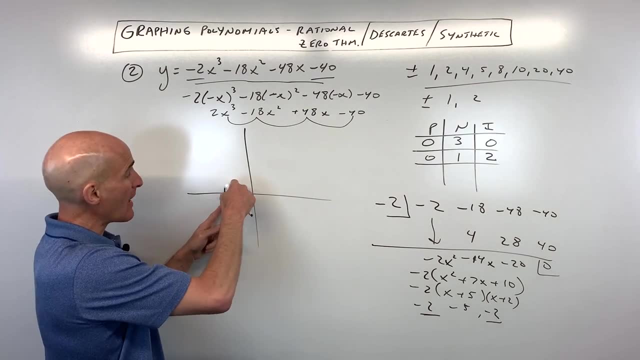 See how we have negative 2 twice. That's what we call a multiplicity. So it's crossing at negative 2.. That's a multiplicity of 2.. It's going to have a, a shape like a parabola shape, either like this or like this when it touches that point. 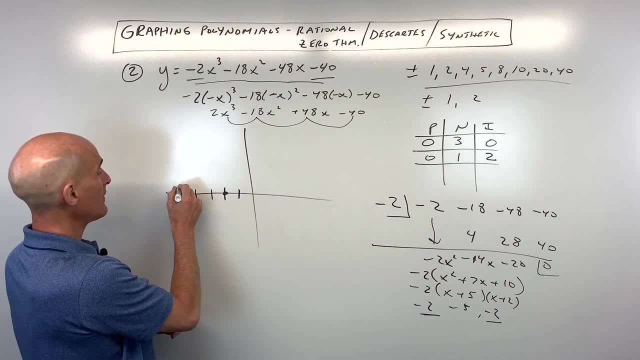 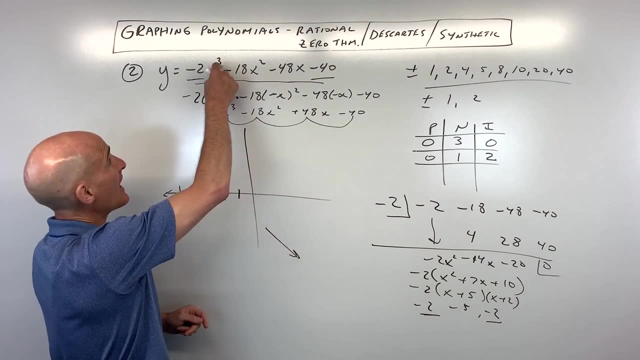 It's also going to cross at negative: 5,, 3,, 4,, 5, right here The leading coefficient's negative. That means it's going to be going down to the right. It's an odd degree, That's 3.. 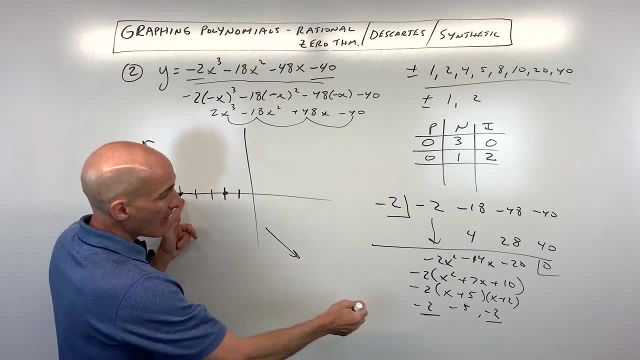 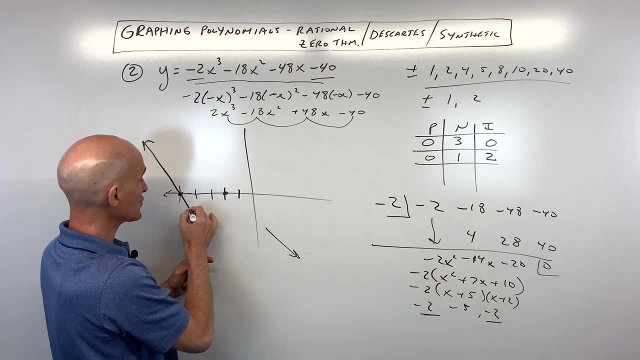 It's going to be going up to the left, the opposite direction, At negative 5, this only occurred once, so that means it's going to go through here just like a line. But here, at negative 2, we said that was multiplicity of 2, so it's going to have that x squared. 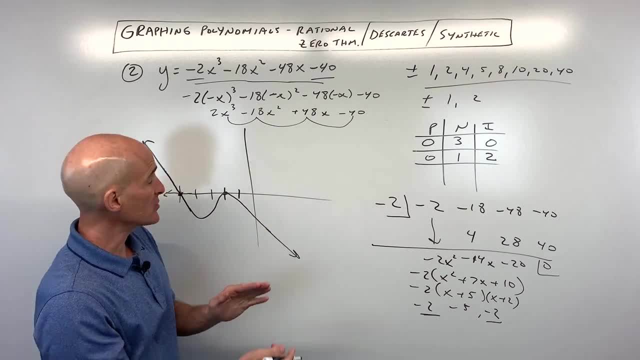 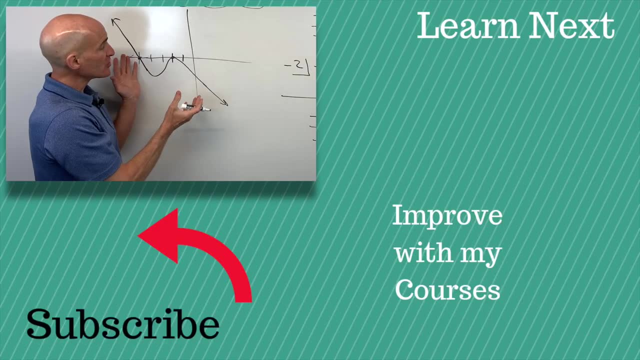 or parabola shape. at that point, The only thing that's missing here is we could pick some points- you know additional points- to get a better idea about how low this goes or how high it goes, But this is a pretty good sketch of our graph, given the fact that you know we weren't. 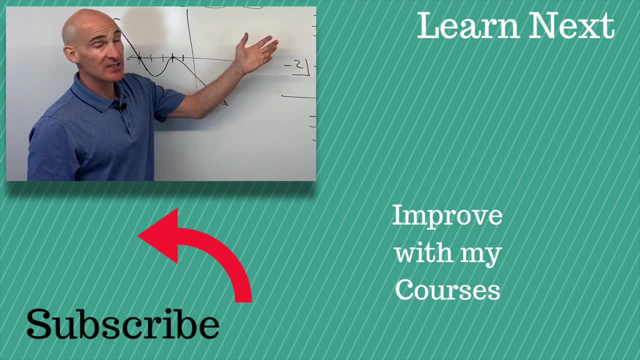 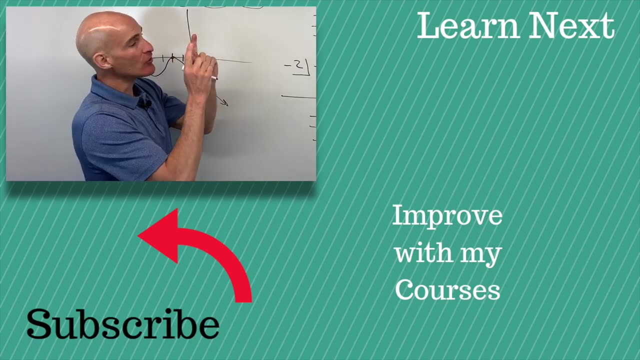 necessarily able to factor it initially, and we had to use a synthetic division and the rational root theorem Descartes' rule of sines. If you want to see more examples like this, follow me over to that video right there and we can dive into some more practice. 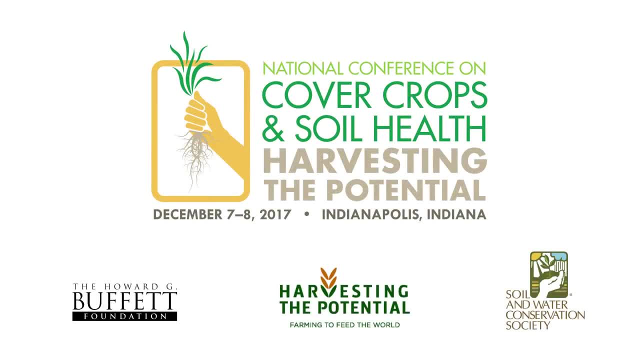 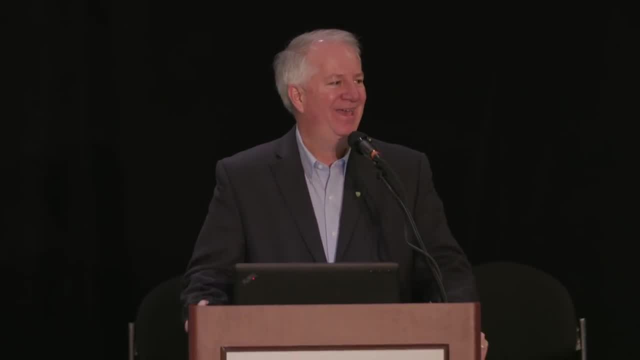 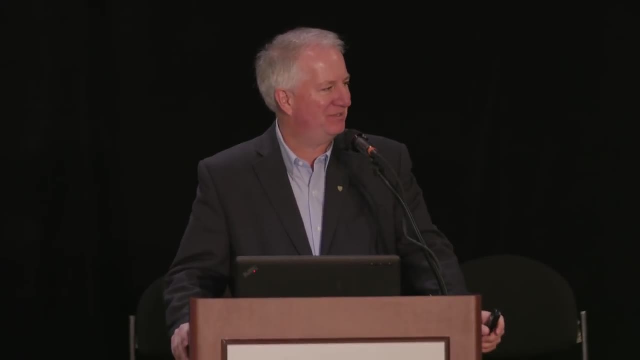 All right, Well, good morning. My name is Rob Myers and I'm with the USDA Sustainable Ag Research and Education, or SARE, program, based at University of Missouri, And I'm pleased to welcome you back to the second day of our conference. We've got more great speakers. 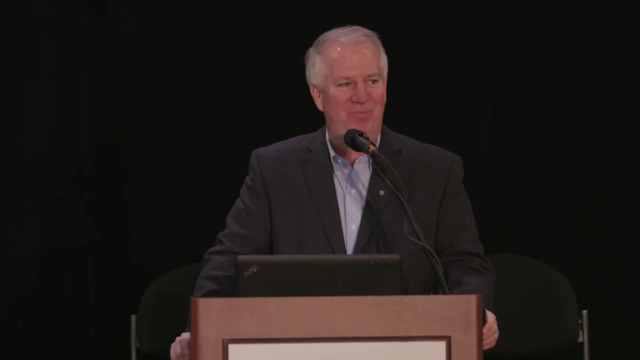 this morning. I'm especially looking forward to Keith Burns talking here in a bit about carbonomics. I've had a chance to hear Keith before and he does a great job. I've got a couple of announcements before we get started. One is that there's still a few seats on the 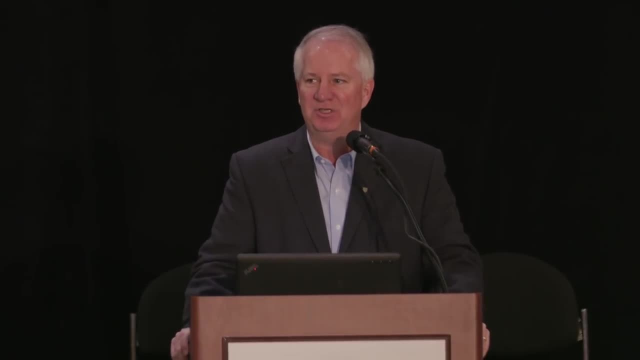 bus tours. So if you're interested in those, you can pop out to the registration area. They told me they can still arrange a lunch if you want to go on either of those bus tours. So just check out at the registration desk right outside the room Also, if you're interested. 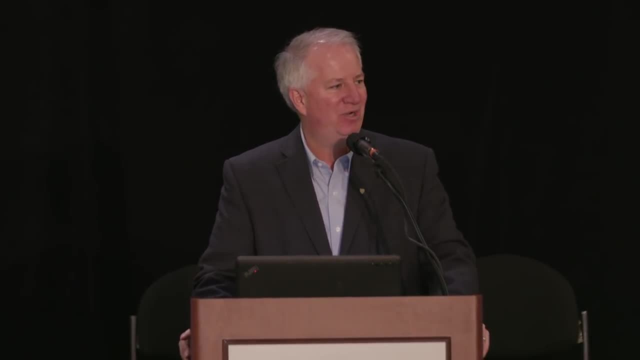 in CEU credits. you can also take care of that at the registration desk. So we're going to have a couple of talks here this morning Before we get into our breakout sessions. following the coffee break this morning I'm kind of the warm-up act to Keith, So I'm going to give you a little bit of a perspective on 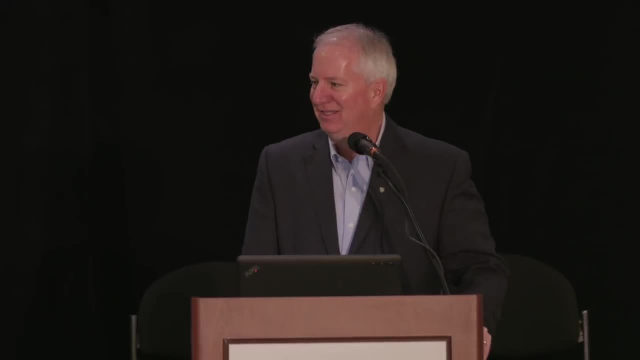 some things going on in cover crops related to soil health, And then Keith's going to take a deeper dive into what's happening down in the ground in terms of the underground carbon economy And, as I said, I've had a chance to hear Keith do this talk and it's 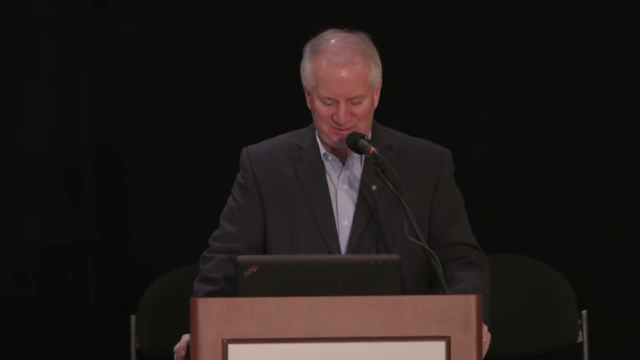 a really interesting and fresh way of looking about what happens in the soil. You know from my own journey with cover crops. I've had a lot of experience with cover crops. Like a lot of you, I got exposed to them early on. We had them on our Central. And that kind of stuck in my mind as a young boy And then years later, when I was starting to do research as an agronomist, cover crops were one of the things I started to work with in the early 1990s when I was working on diversification of crops, And I've had a lot of experience.